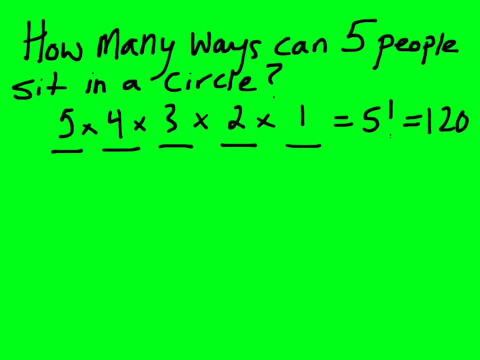 Three, two, one. So there'd be 120 arrangements possible for the people to line them in that line. However, in a circle it's a little bit different. Let me just draw you a couple of examples. So if you have five people sitting around a circle, one, two, three, four, five. 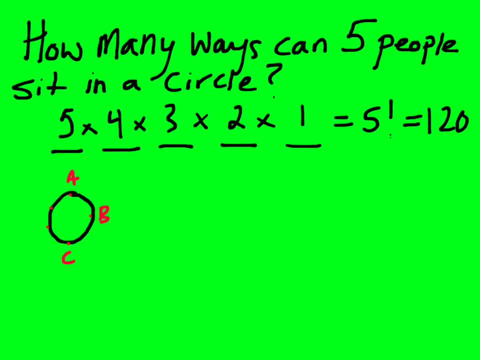 So let's just call them A, B, C, D and E. Well, if I draw another circle and I can sort of have the same kind of idea: one, two, three, four, five, A, B, C, D and. 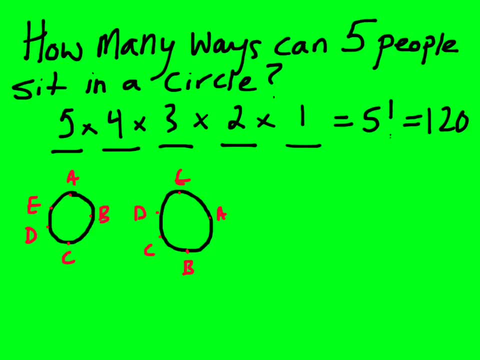 E. So you sort of get the idea that these arrangements are kind of the same. They're not. they appear to be different, but the relative position of the people haven't changed. So A is sitting next to B and A is sitting next to E. It's the same thing over here. 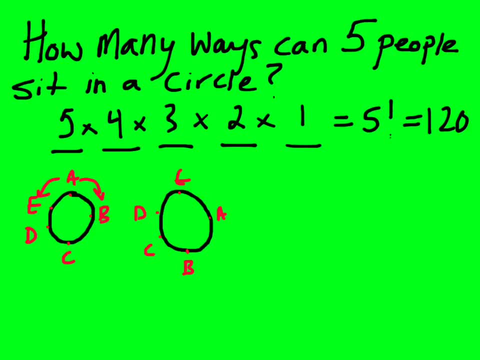 A is sitting next to E and A is sitting next to B, So it's just the same right here. So you can actually do this, of course, five times. So, in order to get this answer, or how many ways can five people sit in a circle? we have? 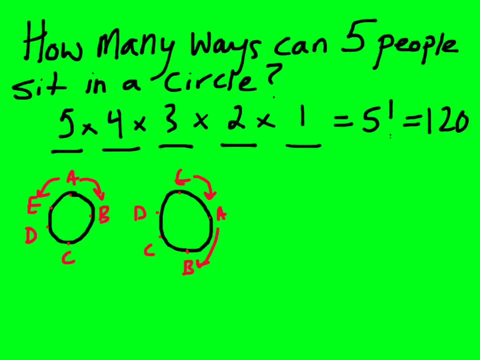 to take account for those repeated arrangements. So what we do in order to do that, we take 120, and we divide by the five possible arrangements that get repeated. So 120 divided by five is, of course, 24.. So that's the way how many ways five people can be arranged to. 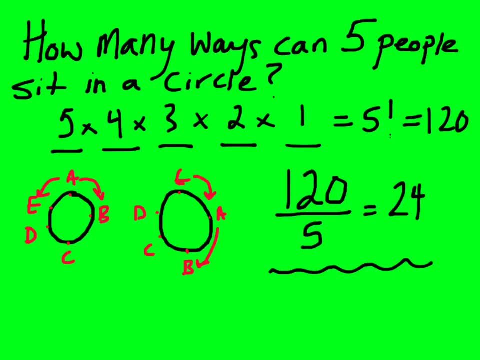 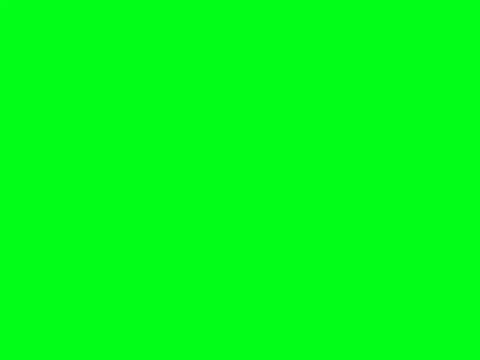 sit in a circle. Now, of course, there's a much easier way to do this question, and that's knowing the formula. So really, the general way of finding this for any value of N is N, and I say N, pick N over N. So in our case that would be five people sit in a circle. 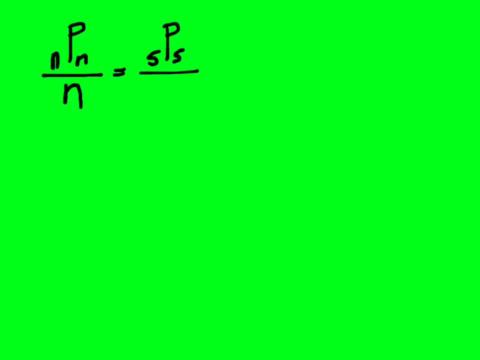 Um, how many ways can five people be chosen to sit in a lot of five And then divide it by N, So that would be just like we had 120, pick five is 120, divide it by five, which is 24.. Now, another way that I like to do this is how I show my students is: